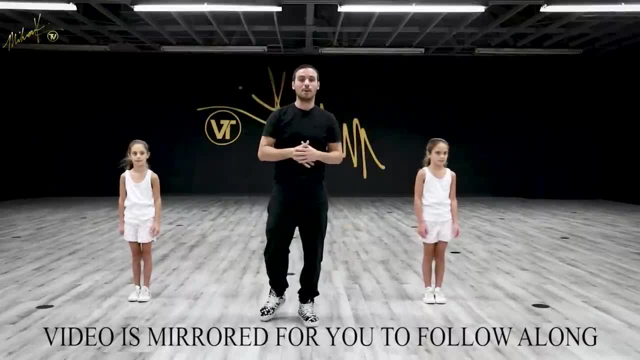 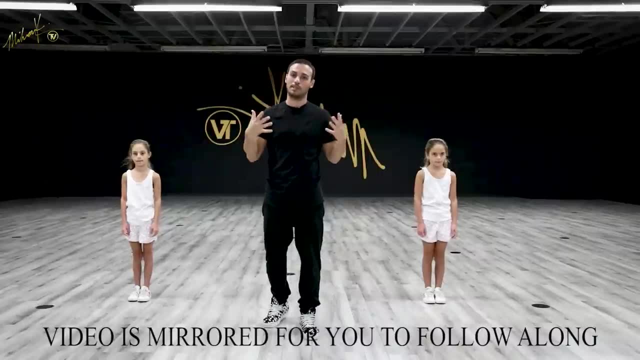 here we go right from the very top. Okay, So, like I said before, we're going to keep the first eight count up and then, on the second eight count, we're going to take it down to the floor. So we'll make sure to do it with music when we're standing up before. 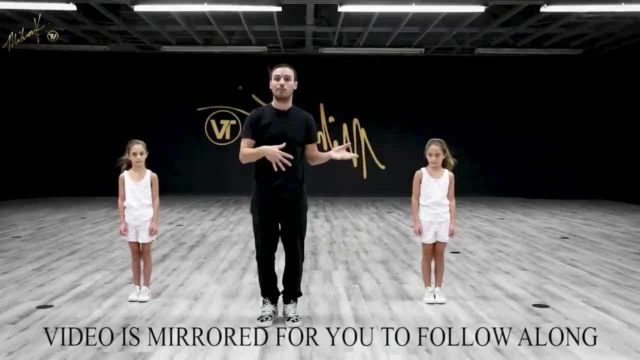 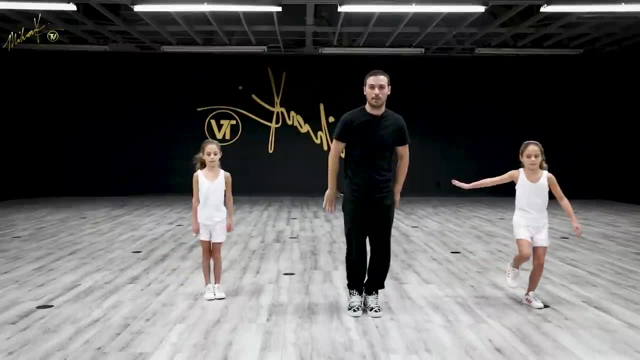 we go to the floor, Here we go. First step is a small little slide. Every time we do our slide, we're going to make sure to come back to our places to start again. Here we go. Seven, eight, We're going. slide two. Perfect, Let's come back again. Let's work. 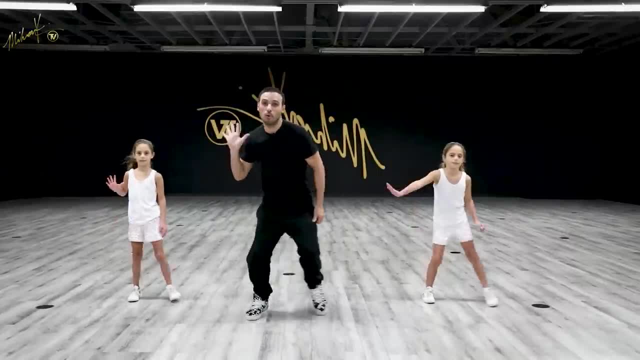 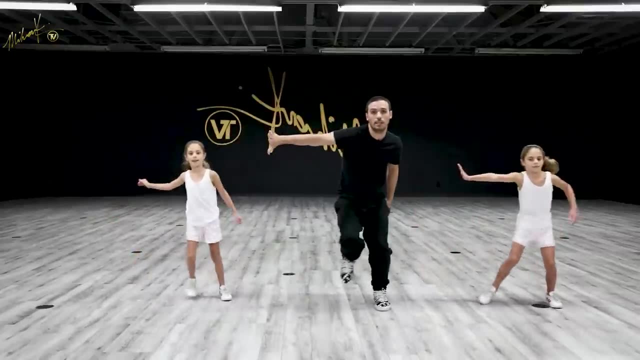 on the slide a couple of times. Six, seven, eight, We're going one, two. Awesome, Let's go again. Here we go: Five, six, seven, eight, We're going one, two. Good, Bring it back. 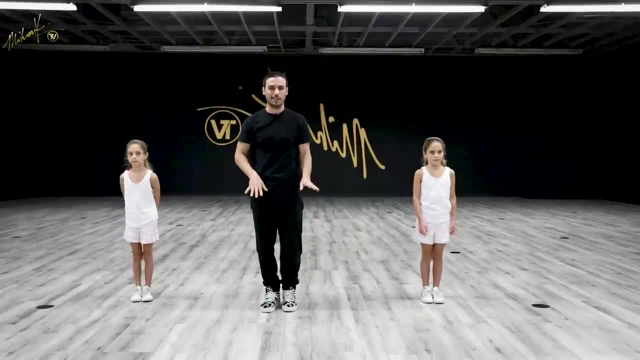 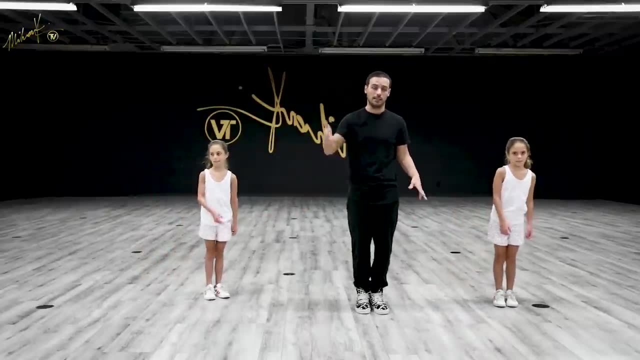 So for the slide, if you've been taking the classes, you already know we've done this. This is a basic slide. We're taking a big step out with the right leg. Whoop, We're sliding the left leg all the way in and connecting, And we're using the arm to look like we're 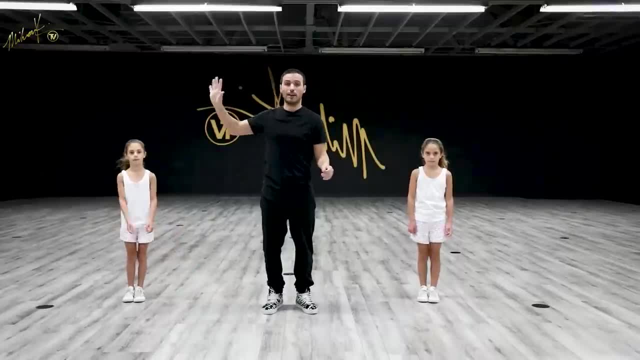 pushing away. okay, So we're going towards the right. We're using the left arm to push away. Yeah, do this, girls. Let's push away. Whoop, whoop. There we go, So lean away with. 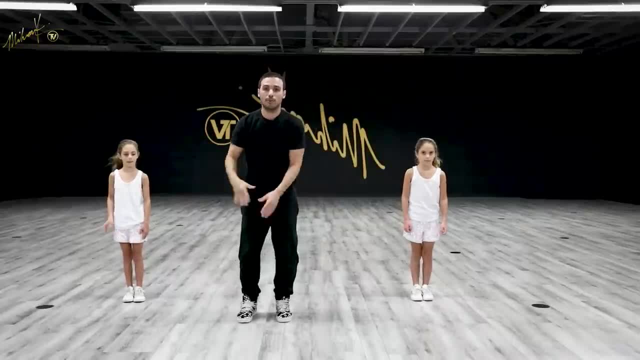 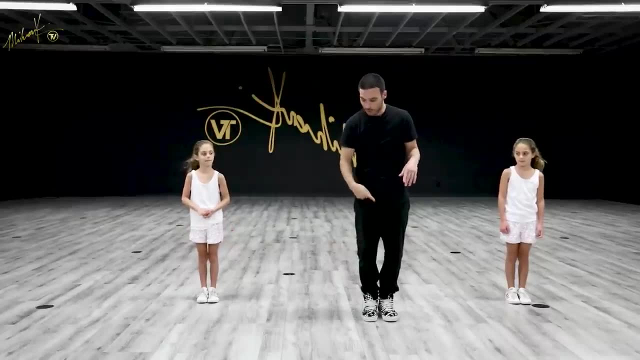 the body, Push away With the arm. Here we go. Six, seven, eight, We're going. one, two From here. once we get here, we're going to do the same exact thing, but this time we're not going to slide, We're. 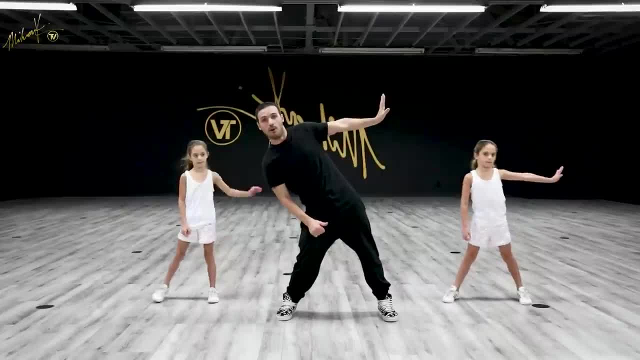 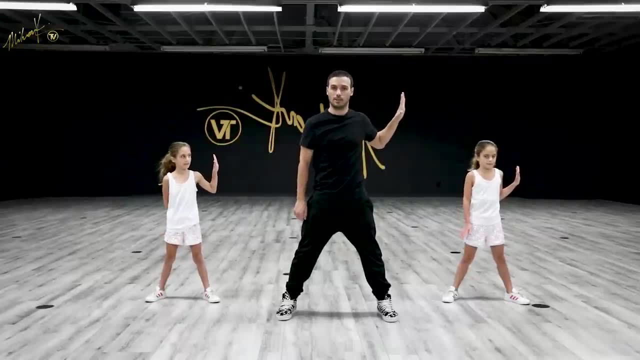 just going to step out with the left leg and push with the right arm. Lean over as much as you can. Put a lot of weight on that leg. Whoop, Bring it back This way. just pull the arm back, just like this. So we're going to step out with the left leg again. Seven: 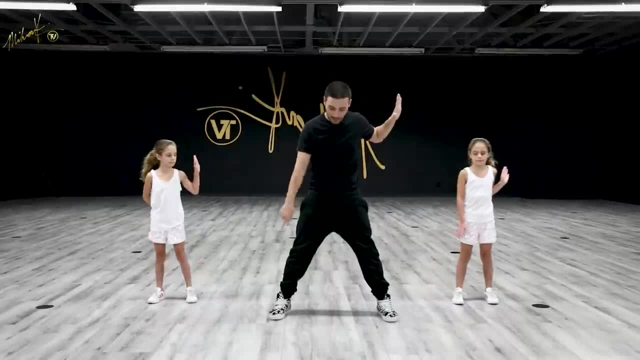 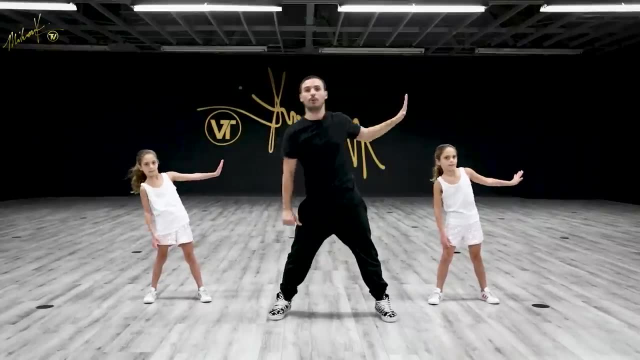 eight: Push and bring it back. Now, when you bring it back, you don't want to move the legs right. We want to keep the legs right here. So it's all about the body. Lean, bring it back. Lean, bring it back. Let's do that a couple of times, girls, just to lean. Seven: 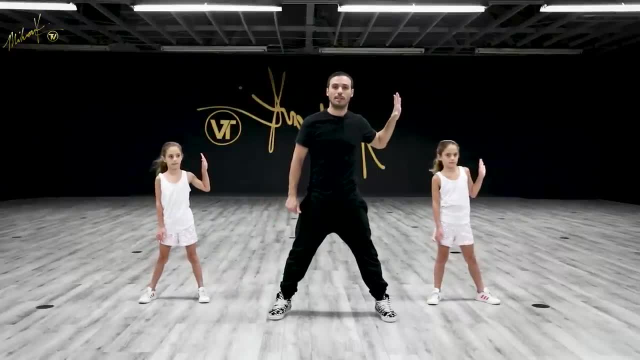 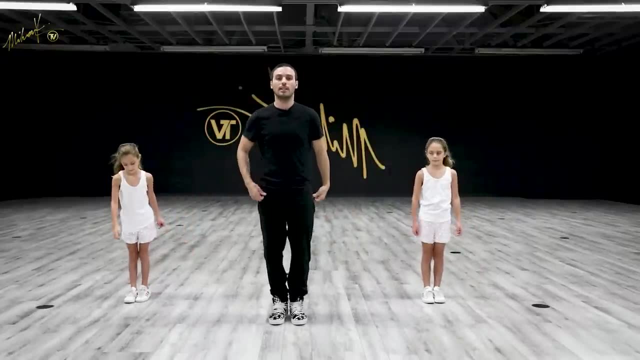 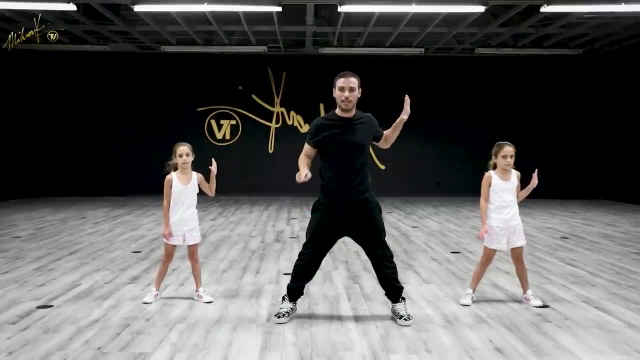 eight. We're going to go lean, bring it back One more time: Seven, eight, Lean, bring it back. Perfect, Let's go from the slide. Let's go from our first position. Here we go Feet together: Six, seven, eight. We're going to go slide and two, Push, bring it back. Good, 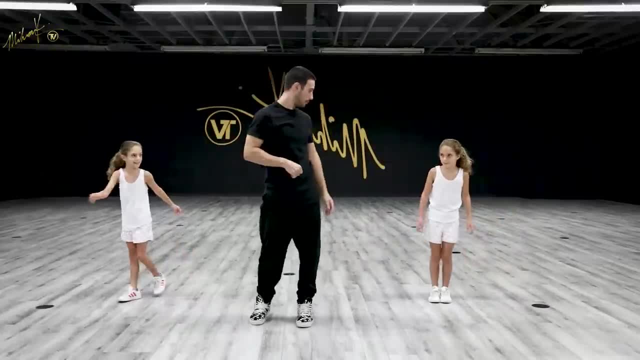 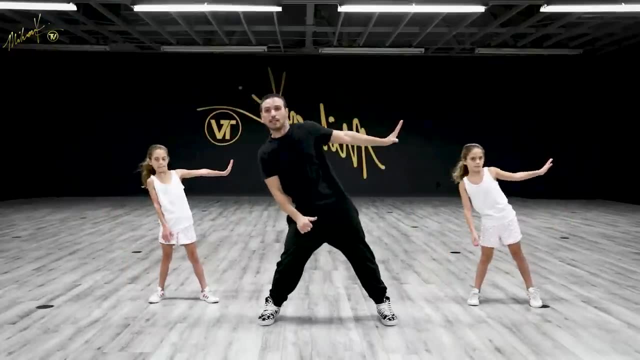 Make sure your feet stay there. Okay, Girls, good so far. Yeah, good so far. Here we go. Five, six, seven, eight. We're going one, two lean hold. Nice, Let's do that a couple of times, see if we can make. 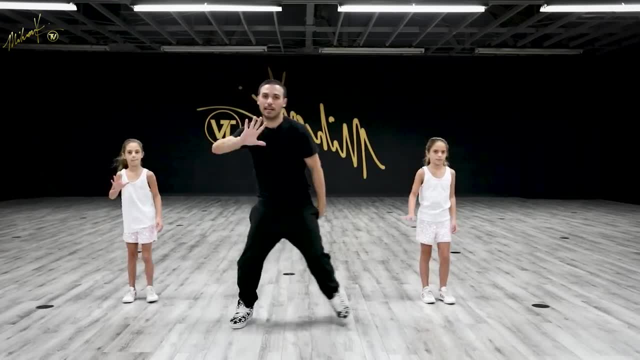 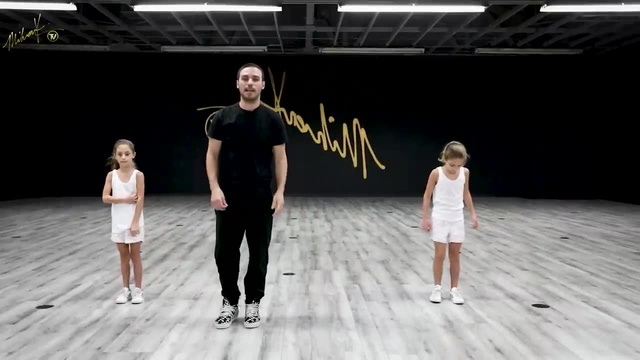 it sharp: Five, six, seven, eight And one, two, three, four. Good One last time. Here we go. Five, six, seven, eight. One, two, three, hold Good Now, moving on to the next. 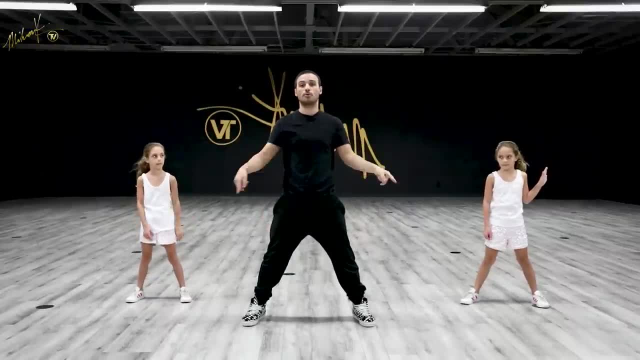 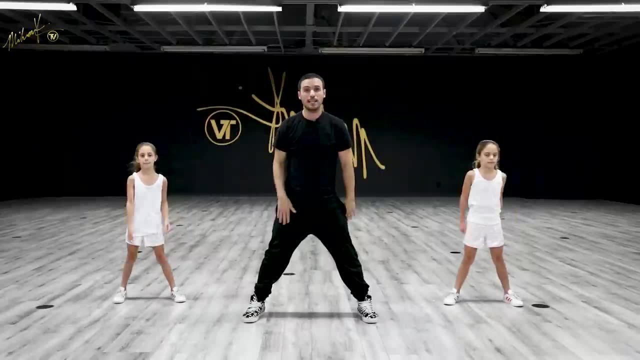 step. The reason our feet are out just like this is because we're going to go into the criss cross step. Okay, We're going to cross the right leg, first Cross. We're going to open up, Woo, And then we're going to cross the left leg. Boom, just like that, Let's go back. 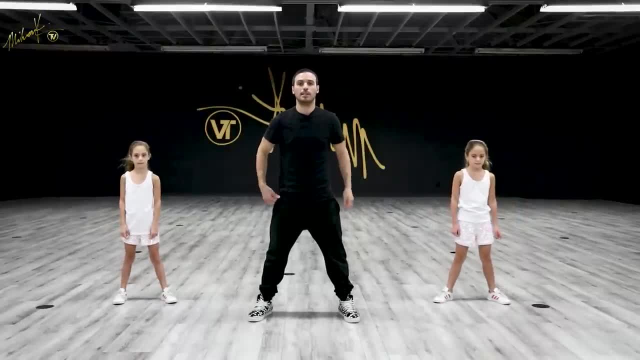 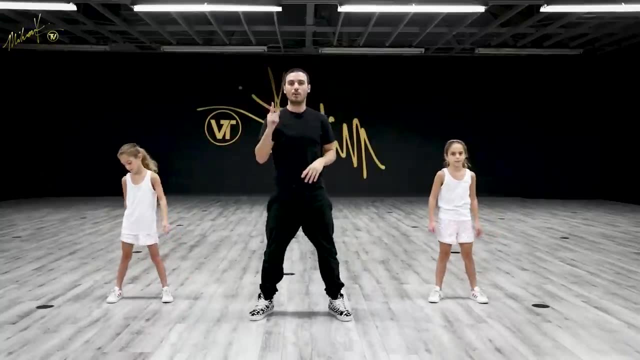 to position one, crossing the right leg first, Six, seven, eight. We're going cross out, cross. Okay, let's do that a couple of times, Just for the feet. always remember right leg first, Six, seven, eight, And go cross out, cross. Don't look for the right leg, You were. 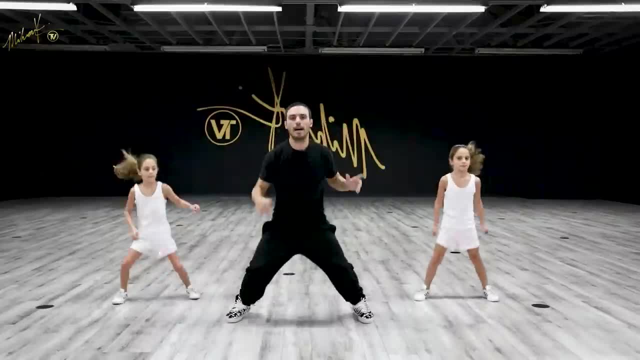 looking for the right leg, not the front foot. You did want to be able to оn that posture and will try and work through it. Six, seven, eight. We're going cross out, cross Cross. Good Girls, so far good. Yeah, Let's end with that left leg and then we'll show them that. 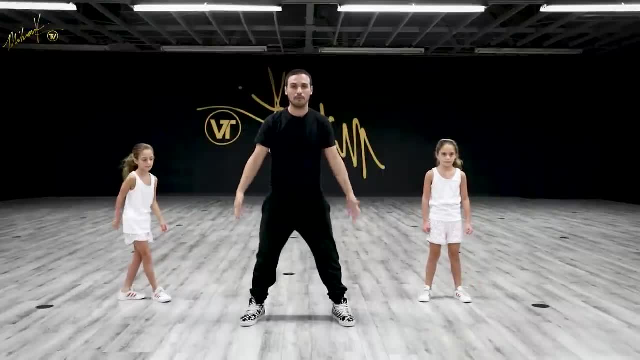 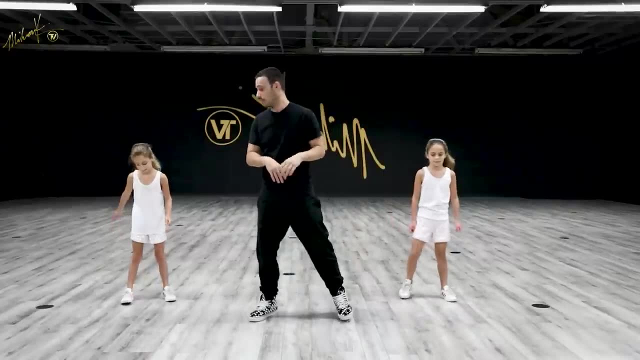 last part. The girls just learned the routine as well. So here we go Five, six, seven, eight. We're going cross open hold One more time. Here we go Five. Let's see if we can do it faster. 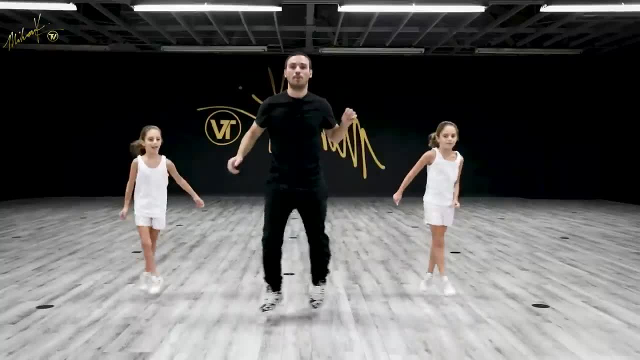 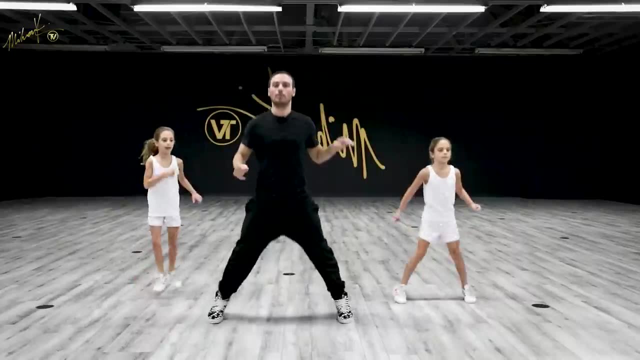 Five, six, seven, eight Cross open hold Good. One more time, Here we go. Five, six, seven, eight Cross open hold Good. Make sure you end with the left leg, Left leg, Perfect Arms, We're going. 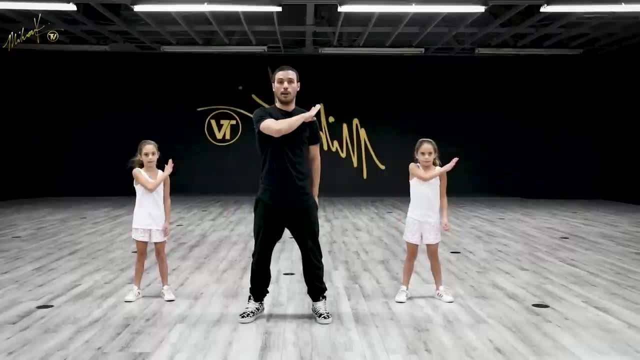 to do the opposite. Let's just show them the arms Girls, we're going to go here up around. and then the next arm: Okay, And we're keeping the arms blades. Okay, Here we go. Six, Just the arms. 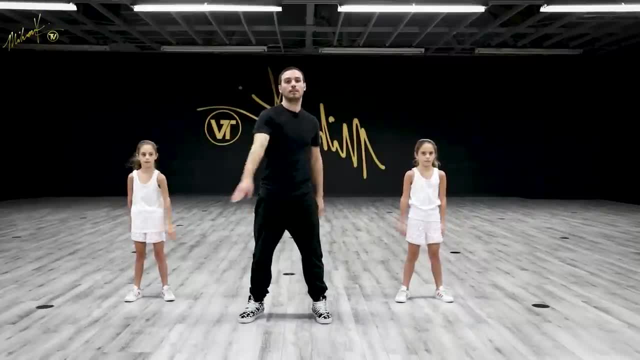 Whoop and whoop, Seven, eight. Whoop and whoop, Seven, eight, One and two, Seven, eight, One and two. Awesome, We want to use these arms with the legs. Okay, Let's do it slow. girls, Here we. 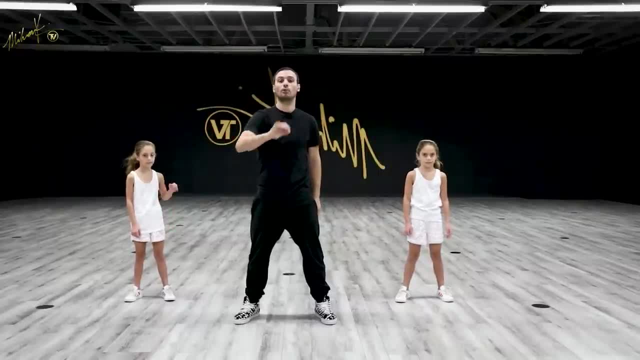 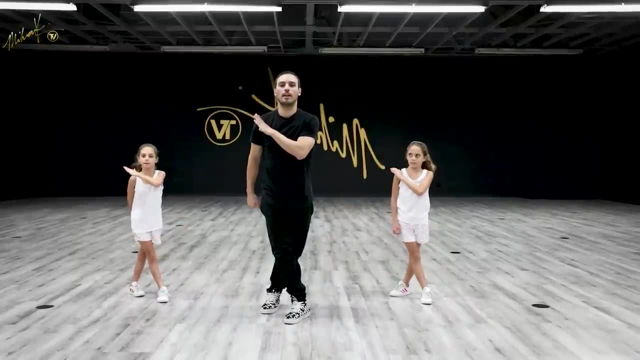 go Crossing the right leg, Bringing up the left arm. We're going to do it super slow, Don't rush. Six, seven, eight, Cross open. cross Good Again. Five, six, seven, eight, Cross open. 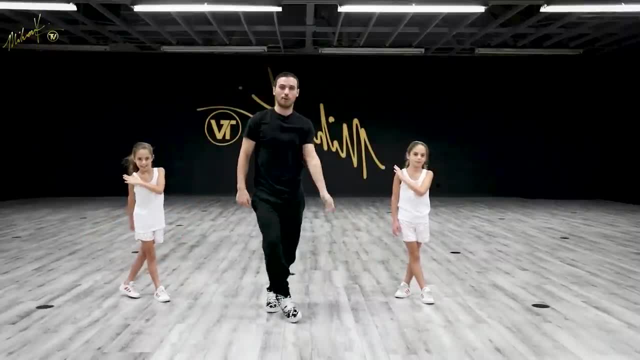 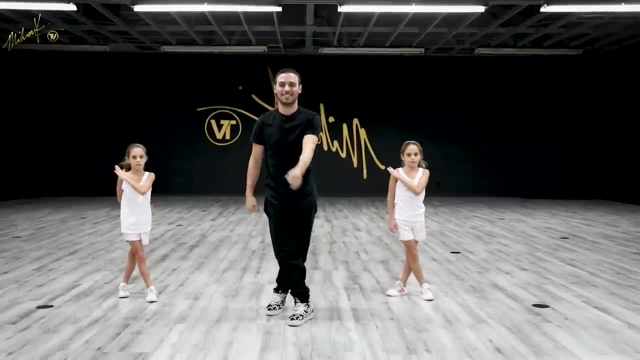 cross Good, Girls working out good. Let's go faster. Five, six, seven, eight Cross open- cross Good. Let's do it two more times like that. Six, seven, eight, Cross open, cross Good. This is. 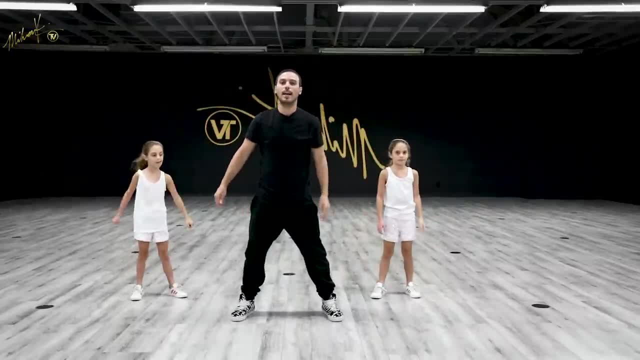 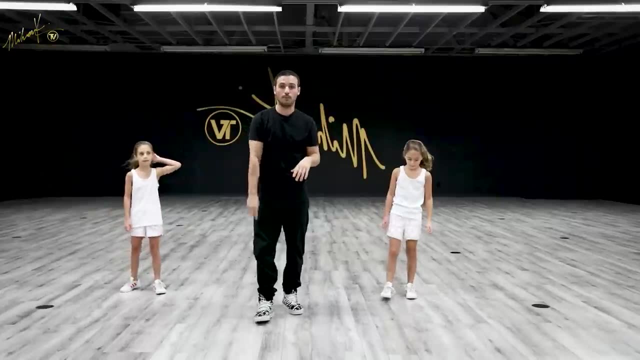 the last one. Here we go, Keep working on it. Six, seven, eight, Cross, open, cross, Awesome, Let's take it back to the very top. Put all of that together. Yeah, Here we go. Five, six from the. 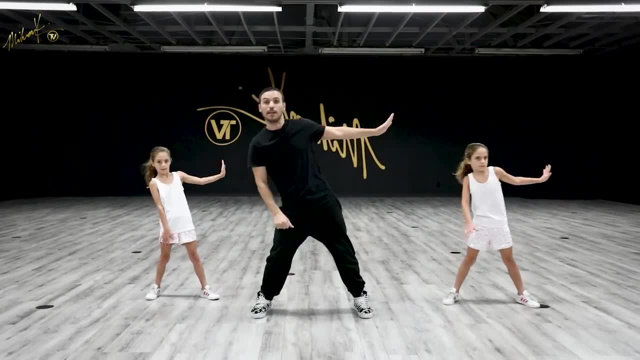 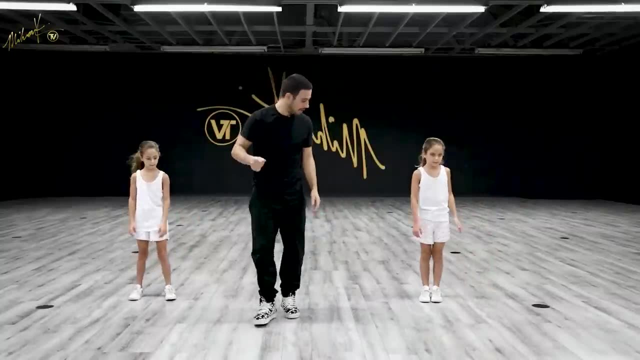 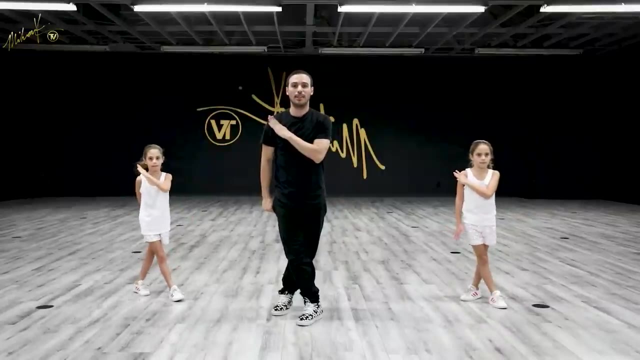 slide. We're going one and two. Lean, come back, Cross and cross. Good, Two more times like that, Here we go. Five, six, You ready, girls, Seven, eight. Let's go. One, two, three, four, Cross and hold Nice One. 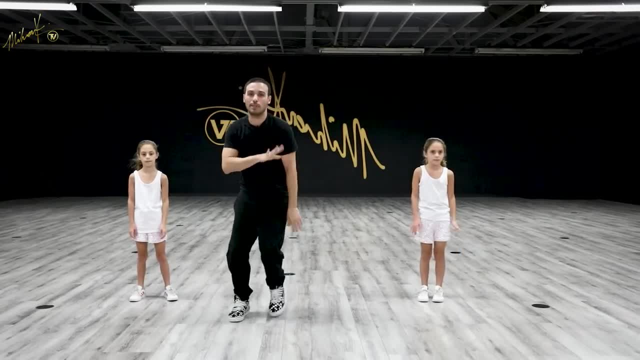 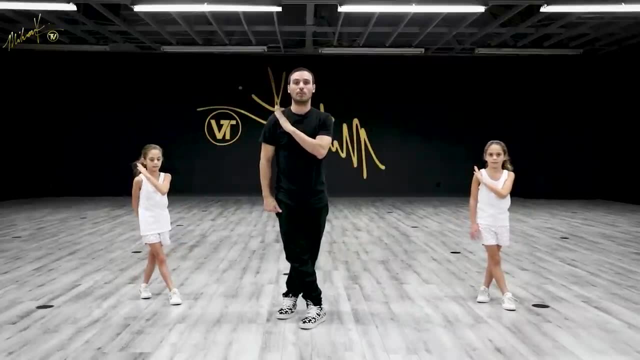 more. We're moving on. Five, six, seven, eight. We're going one, two, three, four, five and six. Let's stay right there, Just to finish up. seven, eight, We're going to jump out. seven Arms are. 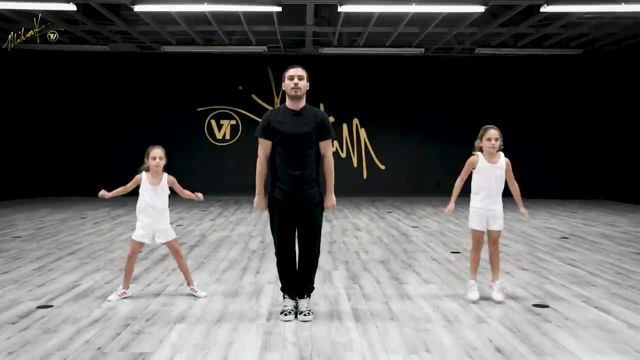 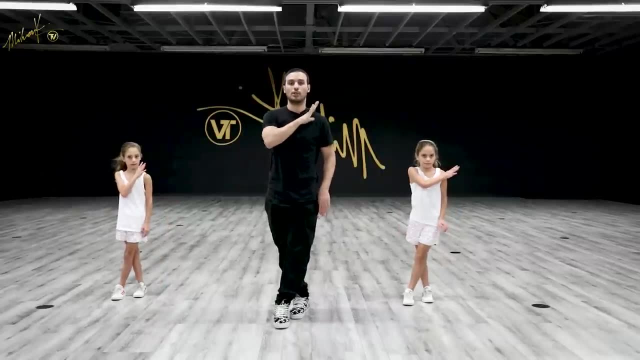 out. Knees are bent a little bit, Lily, Yep, Together eight. Let's try that again. Just the last part. Right leg is in front, Left arm is up, just like this, And we're going to jump out, push the arms out. Okay, Six, seven. 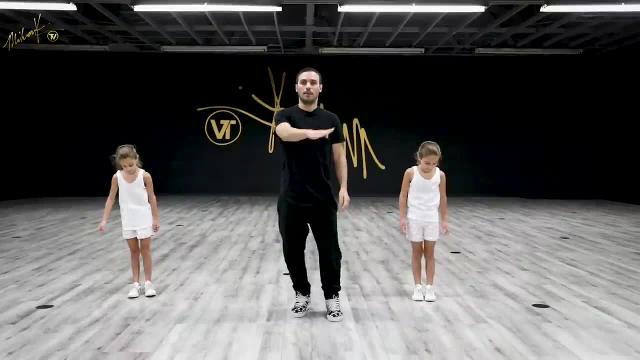 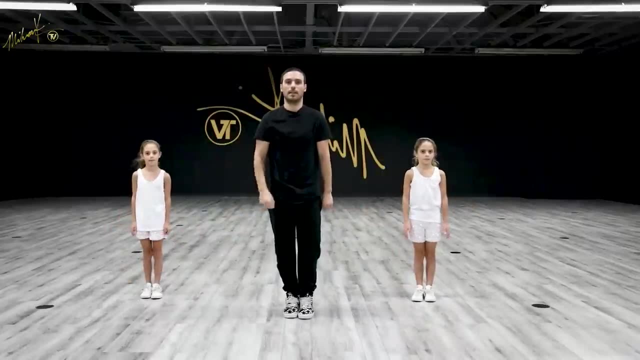 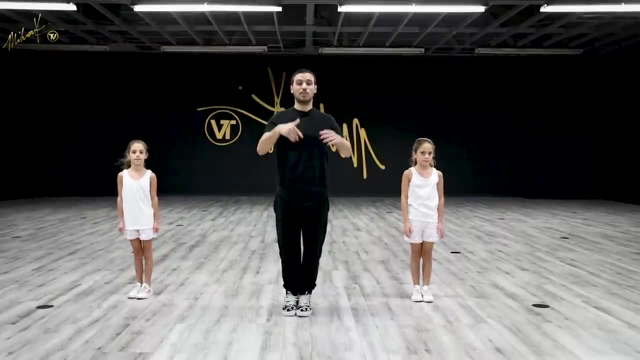 eight Out Together Again. Right leg in front, Left arm up- Five, six, seven, eight Out Together Again. just like that: Five, six, seven, eight Out Together. Perfect, We are done with. 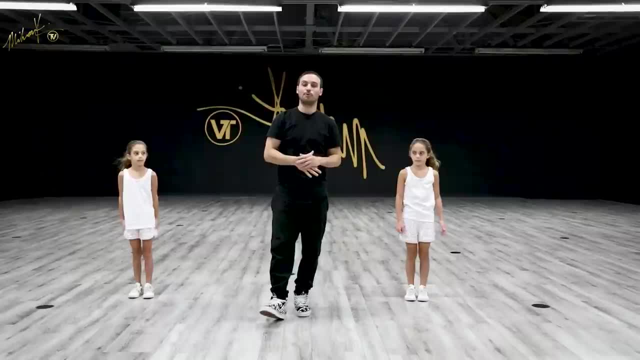 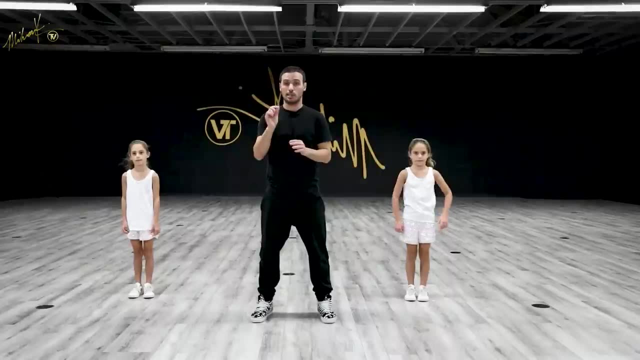 the first eight count. Okay, Second eight count is going to be down on the floor, So let's do a quick recap of the first eight count. One thing we need to remember is when we do the cross, cross and cross, there's a little hold And 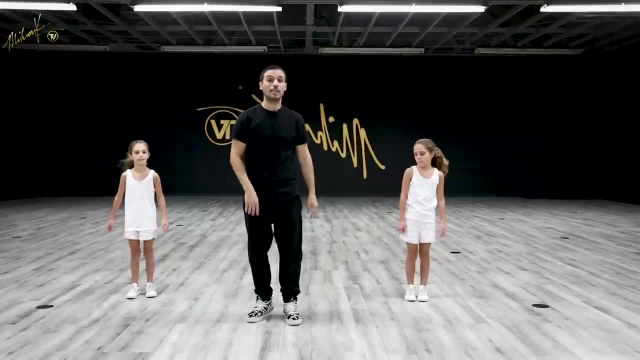 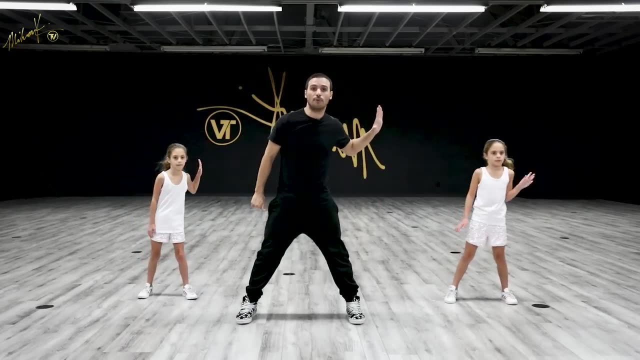 then we go jump, jump. Okay, Let's show them girls from the very top Five, six, seven, eight. We're going one and two, three and four, Cross and cross Out Together. Good, Let's do that. 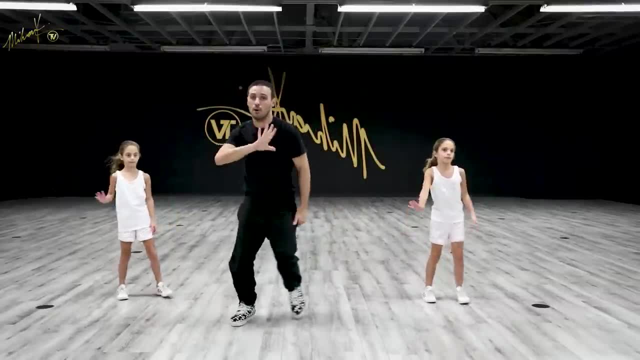 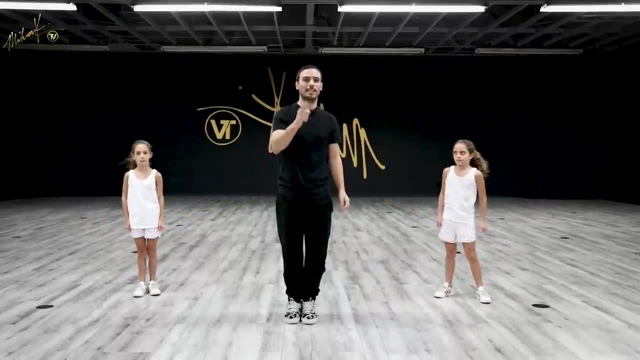 again: Five, six, seven, eight Go. one, two, three, four, five and six seven eight Out. Good, Let's speed that up one more time, and then I think we could try music. Okay, Five, six, seven, eight Go. 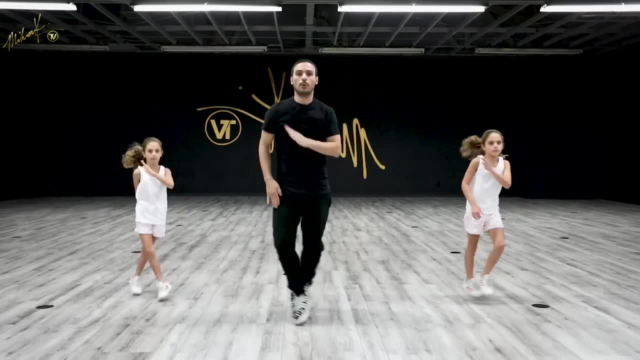 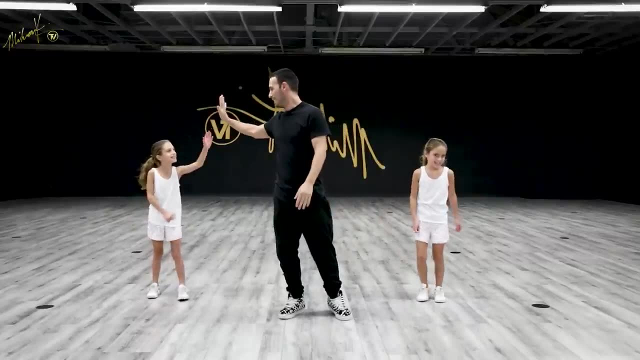 one, two, three, four, boom, boom, boom Out Together. How's that Soft, Good, Good, Mm-hmm Lily, good, All right, Awesome, Let's do it with music, guys, Here we go. 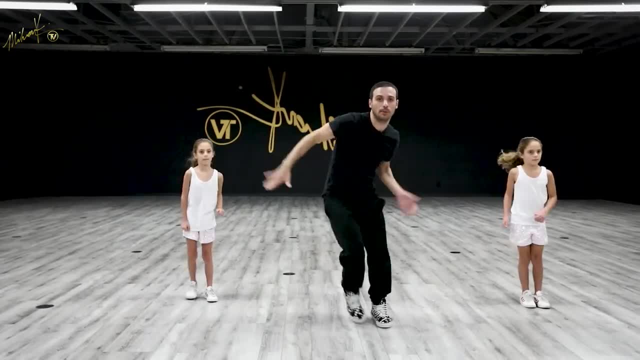 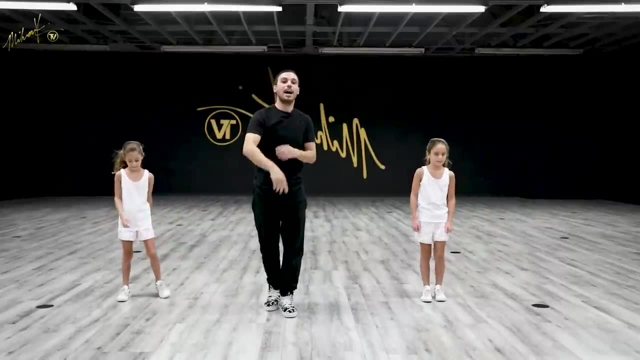 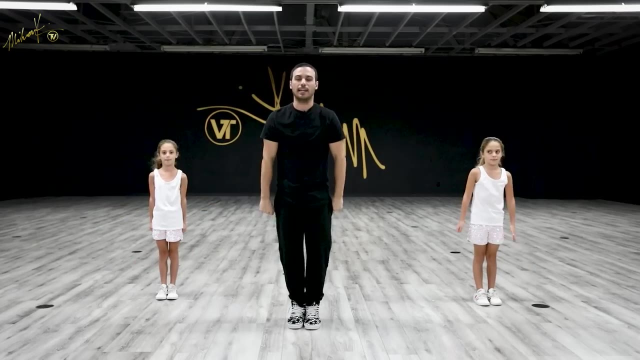 Five, six, seven, eight. One, two, three, four, five and six, seven. Hold Good, Good, Good, here we go again right away. five, six, seven, eight go slide. two, three, four, five and six, seven, eight. 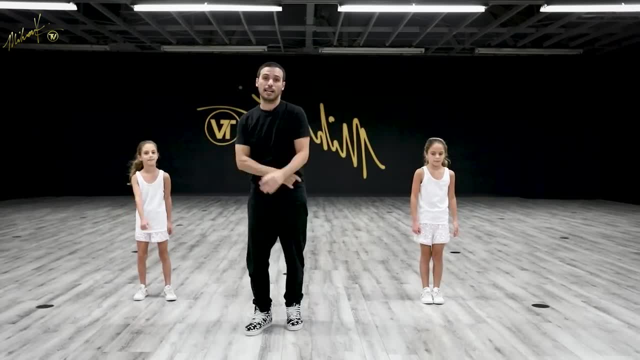 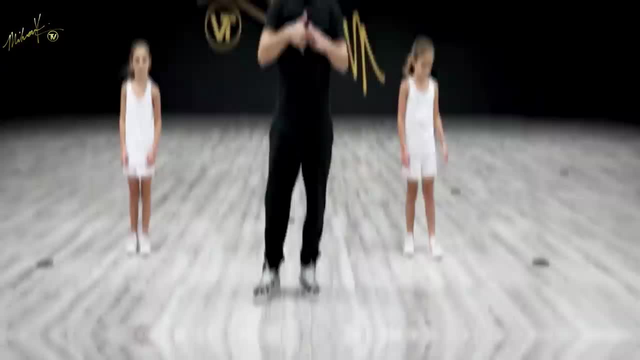 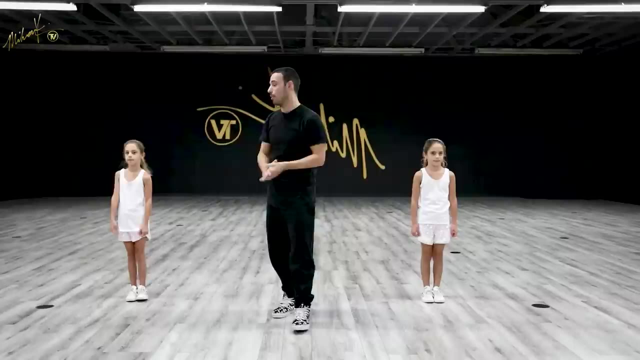 good, let's keep doing it one more time. and five, six, seven. let's go and slide. two, three, four, five and six, seven, eight. all right, awesome guys. that was the first part. let's review it one more time and then take it to the second eighth count, which means we're gonna go down to the floor. girls, one. 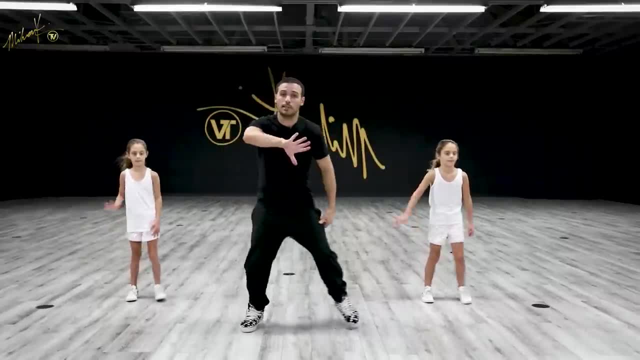 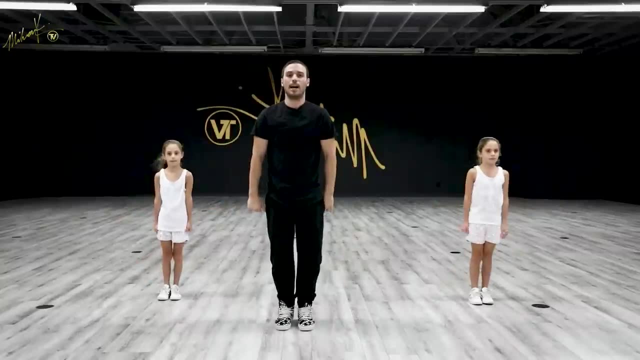 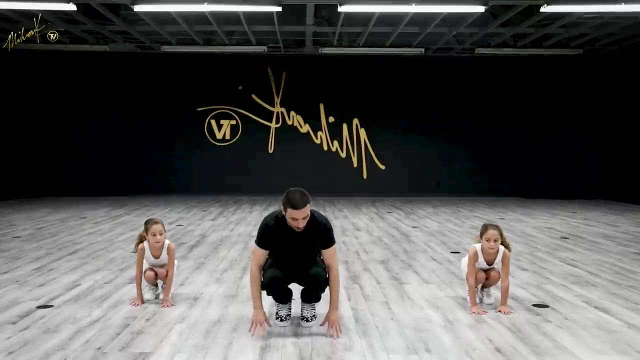 more time from the top. six, seven, eight. we're going slide. and two, three and four, five and six, seven, eight. awesome from here. count one easy. all we're gonna do is go down on count one. that's it. put the arms here, make sure you feel safe. let's come back up. six, seven, eight. one good one more. 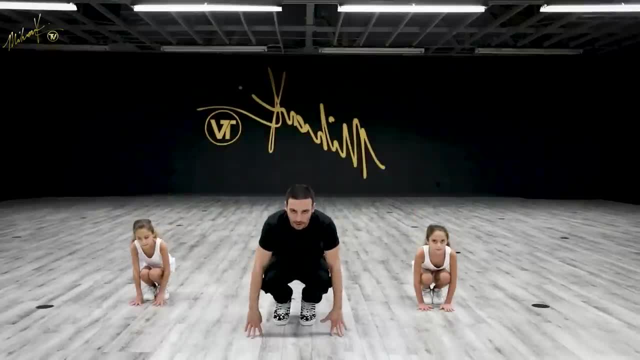 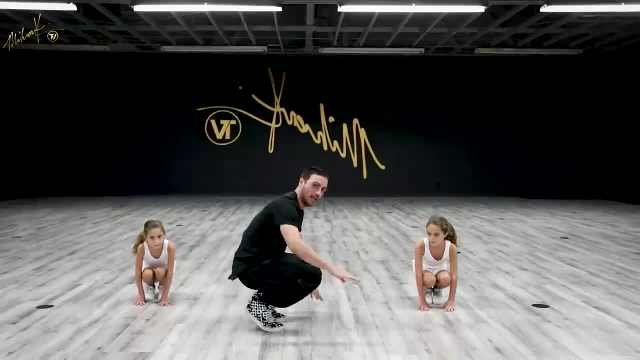 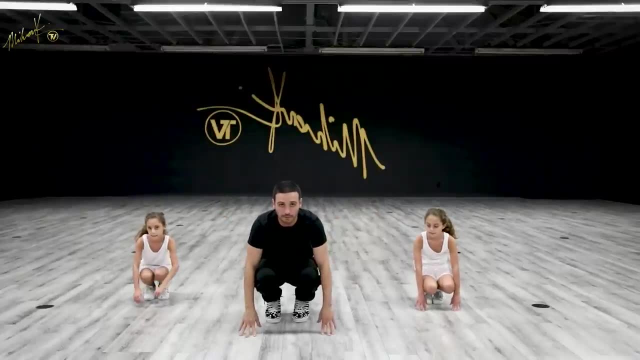 toes. you do not want to come down like this. you will fall to the back. all right, if you're on your tippy toes, you should be able to hold your weight even without the arms. we're going to keep the arms down for safety, but just keep in mind, all you got to do is be on your toes to have a good balance. 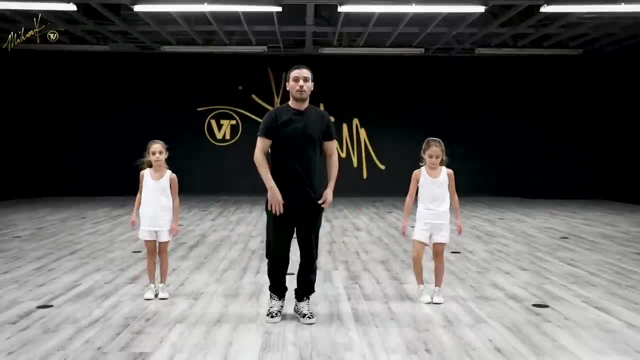 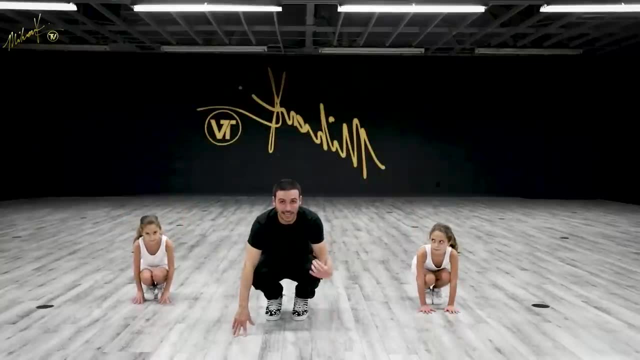 and you're good to go. okay, one more time. girls, here we go. we're going to go down on one and i'm going to show you guys the next move. six, seven, eight down one from here. we're going to kick the legs back and we're going to stay on the tippy toes. you don't want. 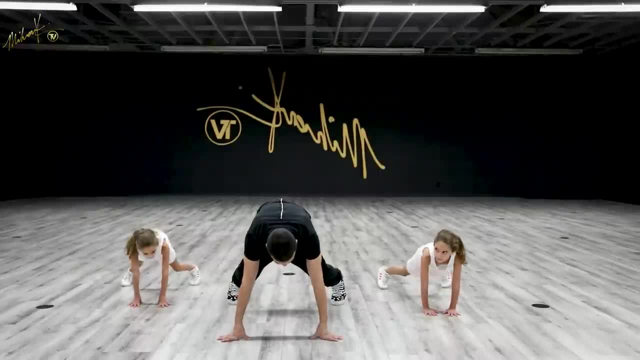 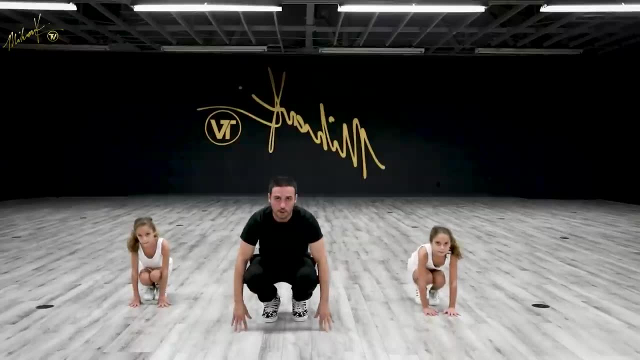 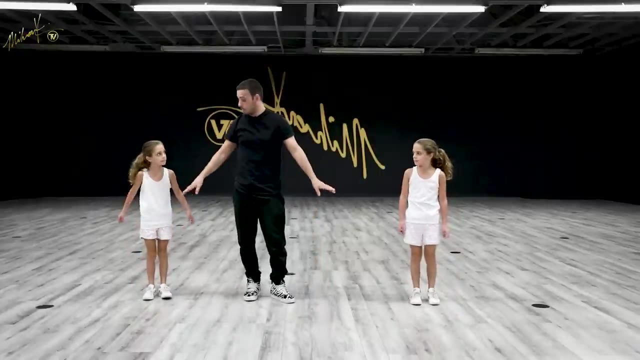 to kick it back all the way, just halfway. two like that. bring it back girls. good job, let's try again. six, seven, eight, two. bring it back one more time. six, seven, eight, two. good, bring it back girls. come on up, i'll have the girls. uh, just stand there and wait for a second. i'm going to show you, guys, what. 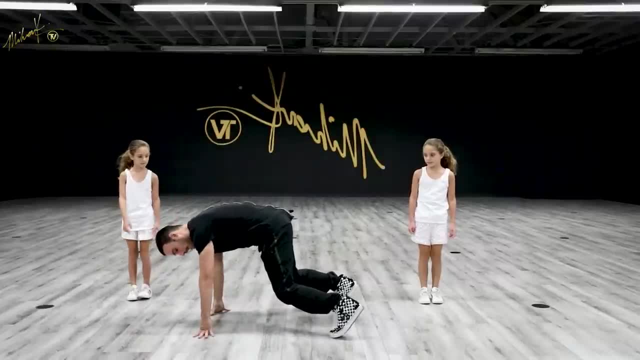 it looks like profile when i kick my legs out. boom, just like that. i don't go all the way out. i'm right here. okay, you're going to kick the legs back and we're going to stay on the tippy toes. you want to make sure you have a good balance. your knees are bent so you can do the next move. 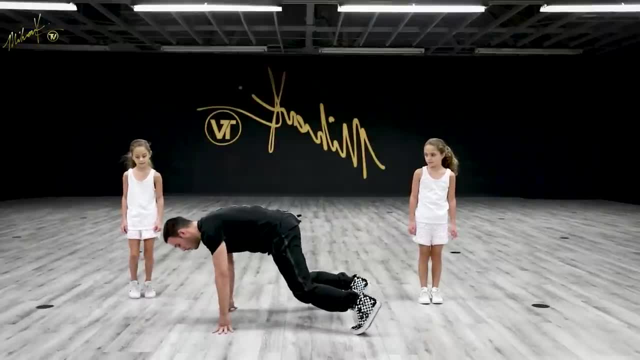 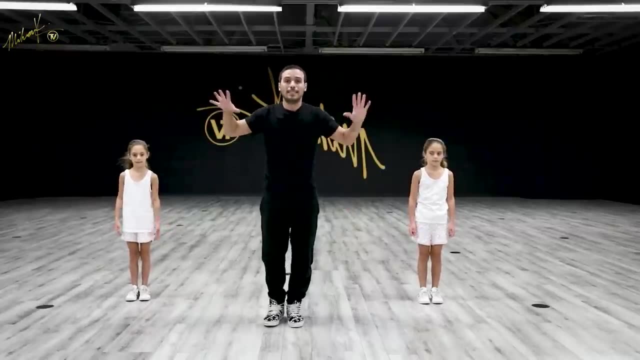 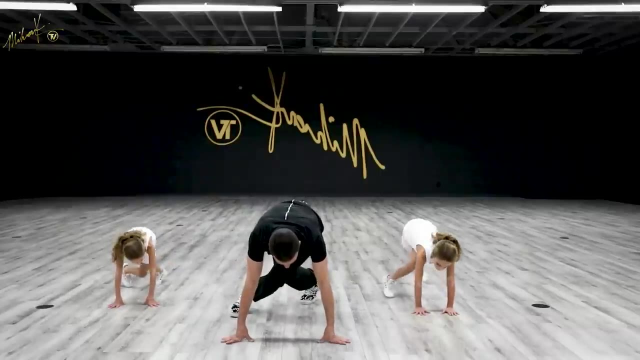 so remember you're here, tippy toes, boom, and that should be good enough. okay, let's do it one more time, girls, and then i'll show you guys the next move: six, seven, eight, down one, legs two. now we're going to do the crisscross the same way: right leg crossing in front, cross open, cross open together. 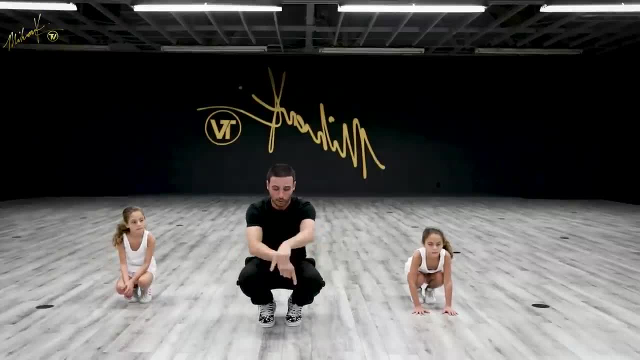 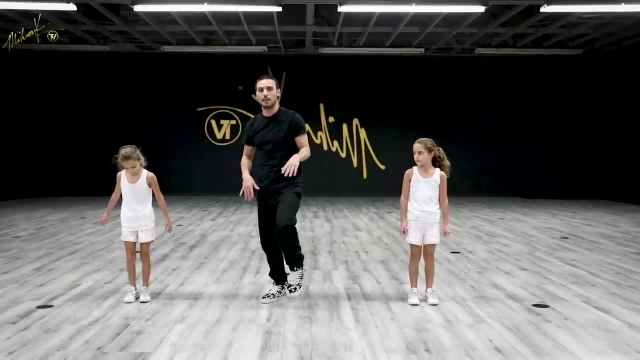 okay, so we just did the same crisscross step on the floor, right open, left open together. okay, let's come back up, because staying down there you'll feel it as well on your legs. okay, here we go. we're going to go down one, kick the legs back on two, we're going to 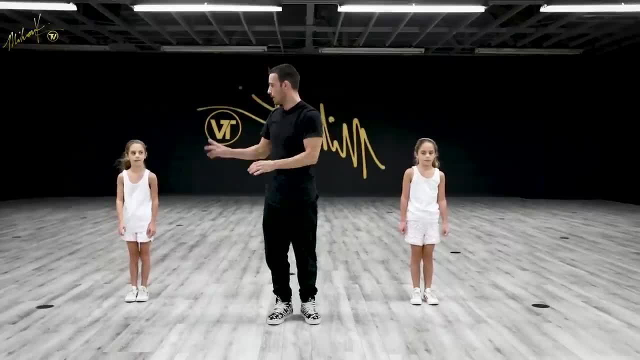 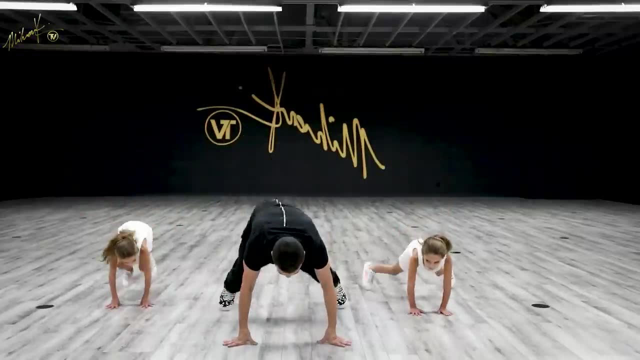 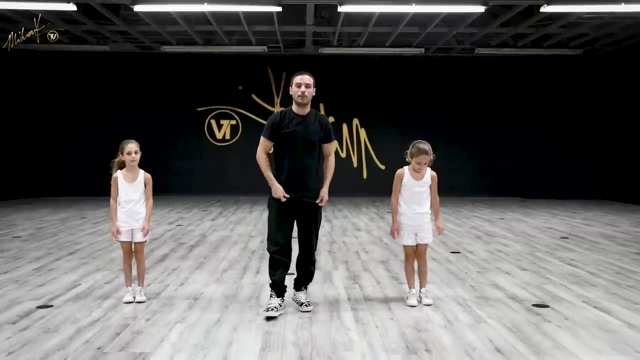 go cross open, cross open together. girls ready, ready, here we go. five, six, seven, eight down. one kick two: cross open, cross open together. good, come on back. let's try that a couple of times, more times. another cool trick during the cross: if you turn your body with the same leg, that's. 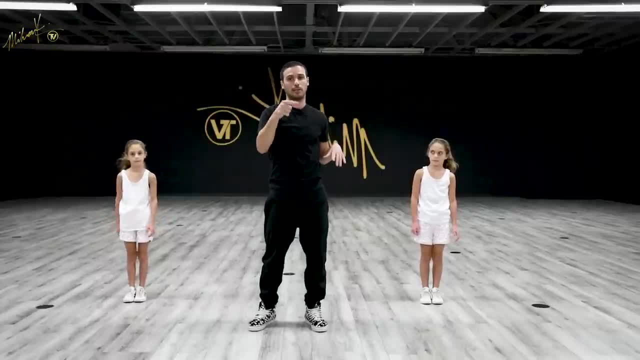 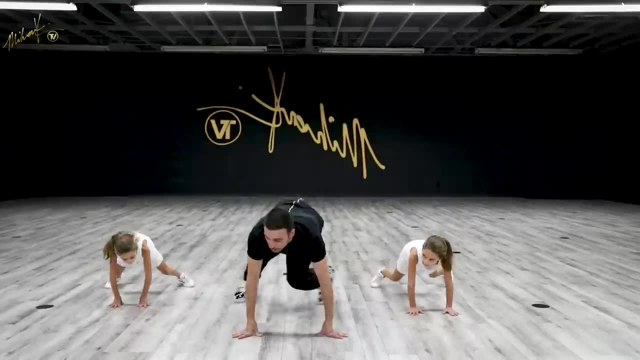 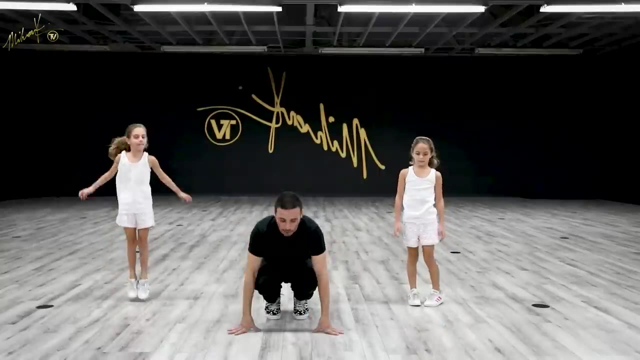 crossing. it'll give you this cool little illusion of you twisting your body. i'll do it this time. you can watch. here we go, girls. five, six, seven, eight down one, two, three and four and five. good, so watch my feet, girls. you guys could stand up for a second. i'm going to show them. 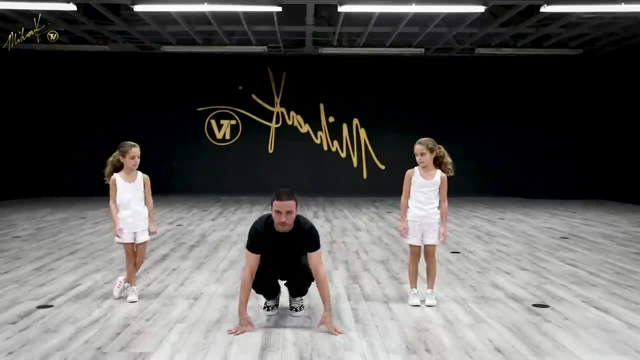 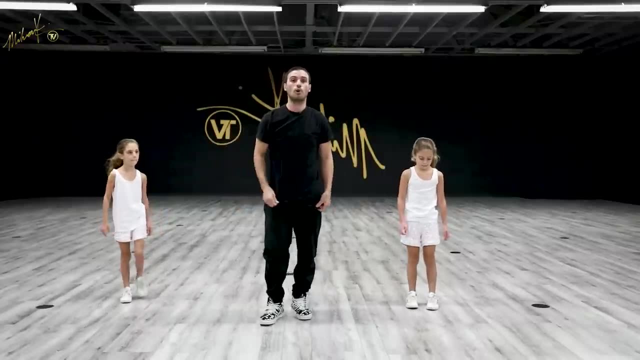 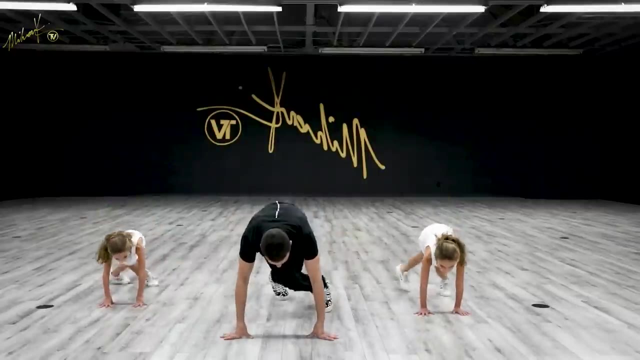 how i twist, i go twist and twist and together so small little twist could change the move a lot. okay, let's do it one more time, and we're almost there. we can finish it up here. we go down on one, five, six, seven, eight down. one kick two: cross open, cross open together. on count five, we have our. 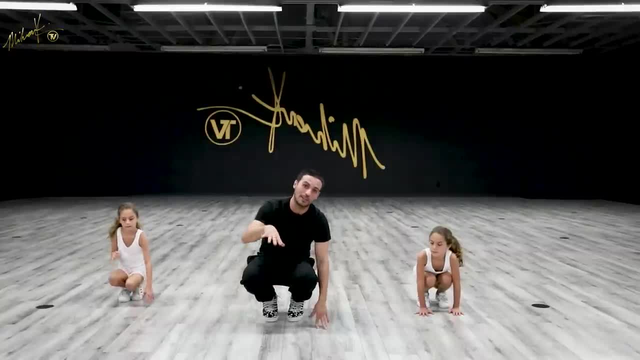 right arm. we're going to take it back on six so we can kick out the legs to the front on seven. so right arm goes here, boom, come back over here again now. it's very important, sophia, because i just saw her legs. we're going to make sure we stay like this. we're going to make sure we stay. 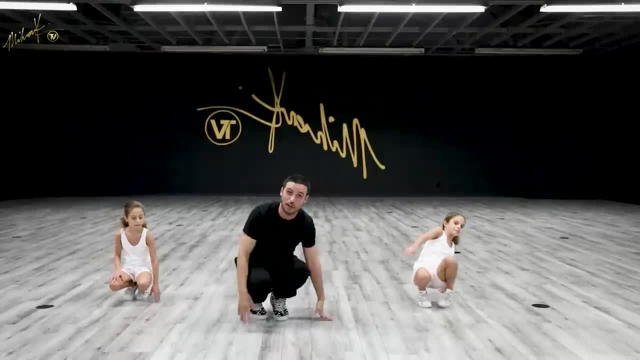 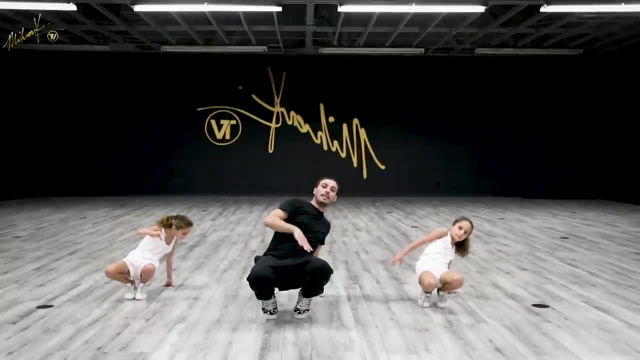 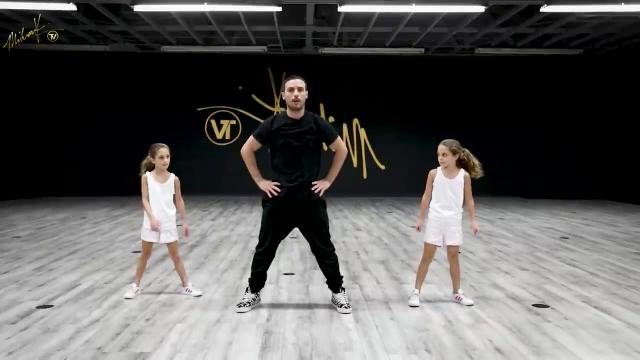 like this, right so? because if we don't, we're going to fall back and it's going to be really hard. so everyone on their toes, right arm back. so whoop, right arm back, lily, awesome, kicking the legs out. boom, bring it back, and then we're going to jump up. good, the girls are going to jump up, put. 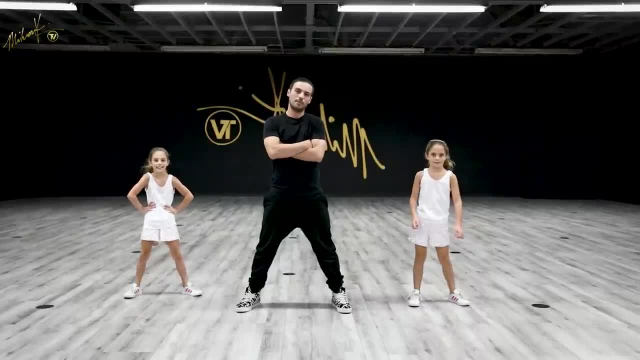 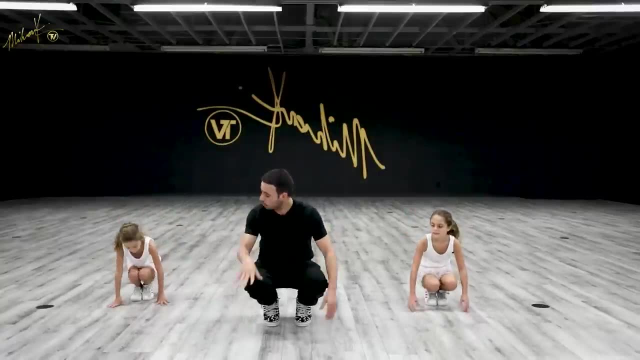 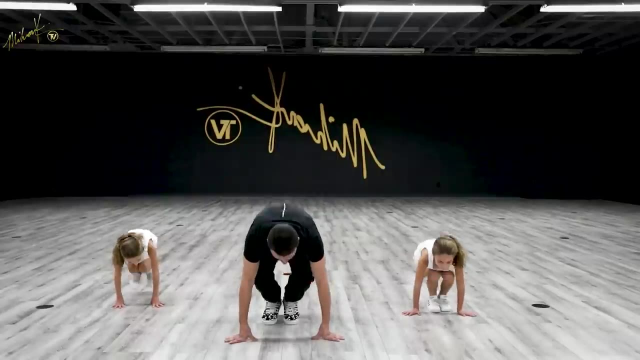 their hands on their hips. right, girls, i'll just cross mine right here, okay, and you decide what you want to do. so one more time. we're down here. this is count one, count two. we're kicking back, we're going to go cross open, cross open together. this is count five. on count six, the right arm goes. 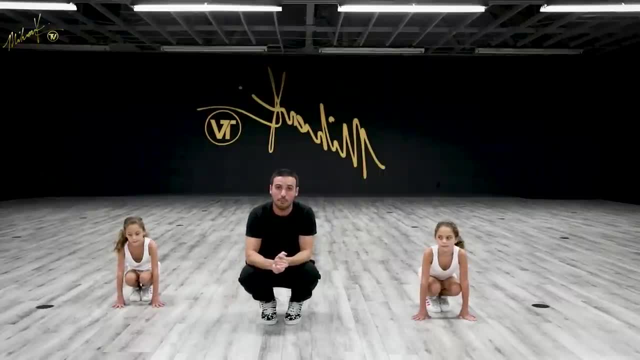 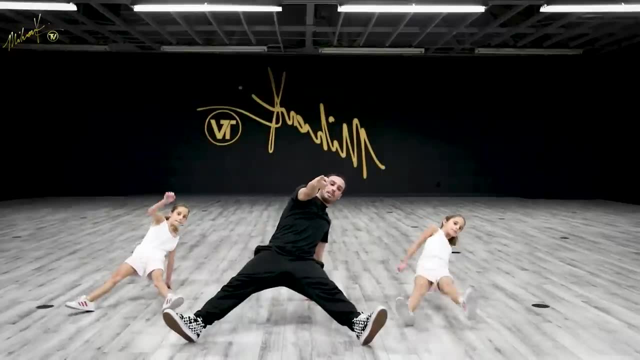 back first because we want to make sure we could hold ourselves up before we just kick the legs out. this is six: kicking the legs out and also the hips up. boom, we're gonna point, bring it back and then we're gonna do our last little jump shoot. i'll be here. 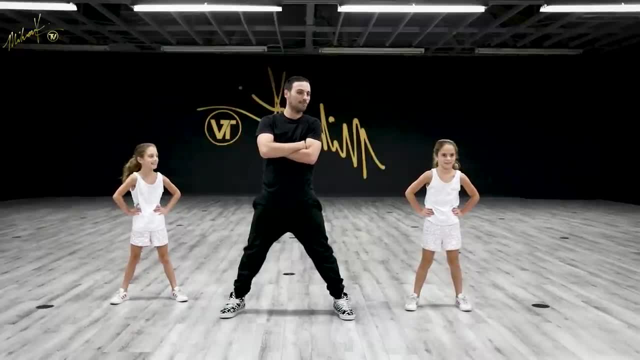 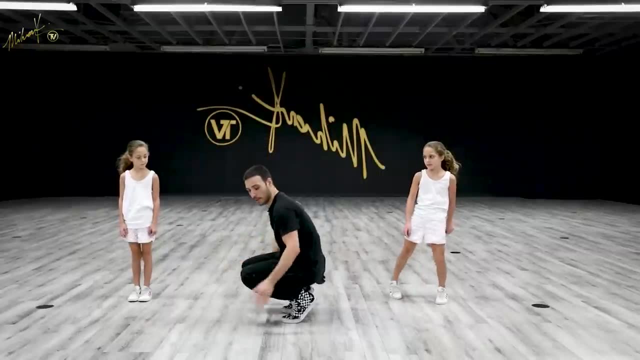 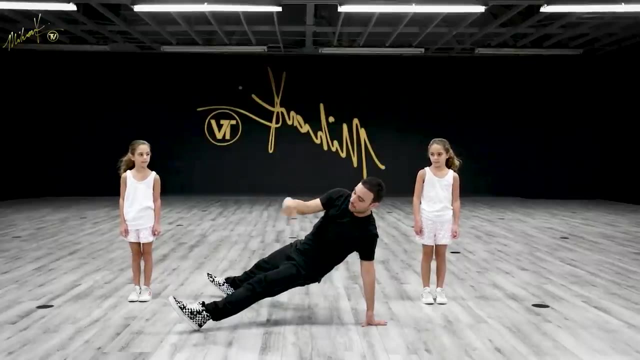 and then lily will be on her hips and sophia will be on the hips as well. all right now. the only other thing left for the kick out is when you kick out, i'll show you profile again. i'm here, my arm goes back six. i do the kick out, boom, pushing my hips up. now you got to do the same. 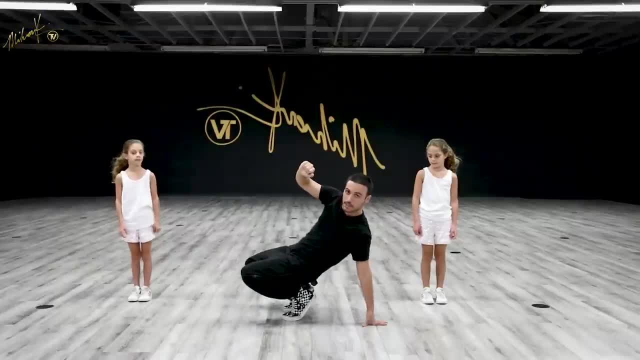 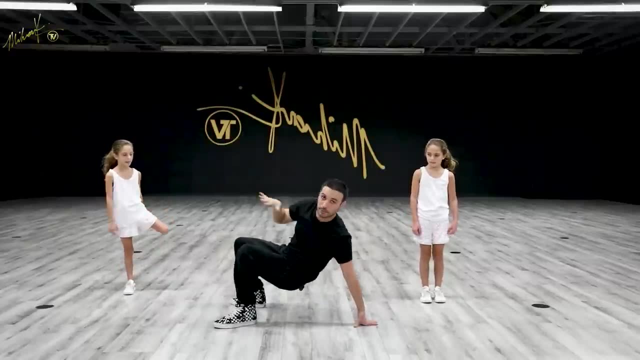 jump to bring those legs back underneath yourself, just like that, so that way you could get out of it. if it doesn't make it all the way down here, you're going to have a hard time. if you get here, there's no way you're going to be able to push yourself back, so out, boom. also. i have a tutorial just on. 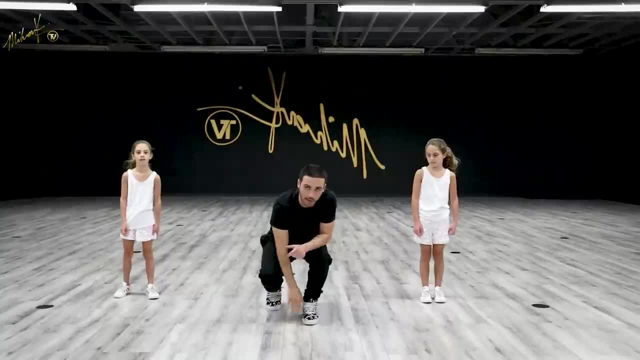 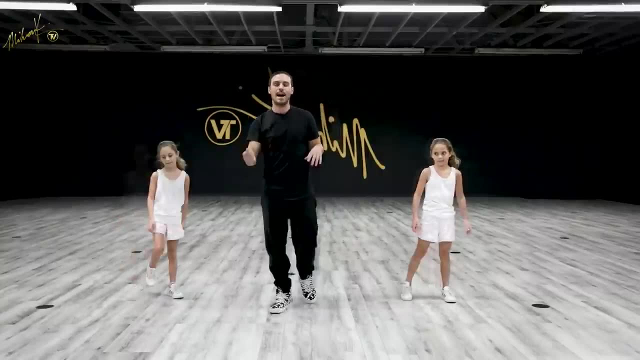 this move, the kick out that i'll put in the description down below if you want to check out description box so you can work on it on its own if you need some time. Girls, should we do a quick recap of just the last eight count Only the floor. Slowly, Here we go. Five, six, seven, eight, Down. 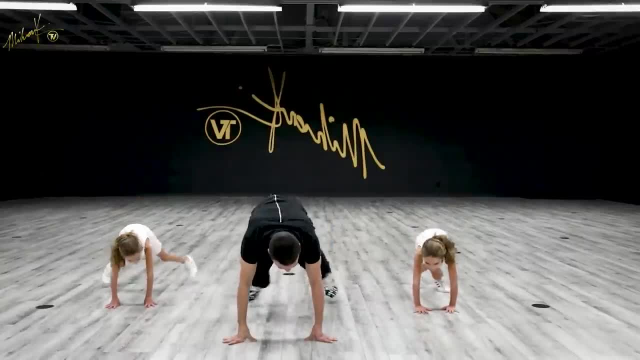 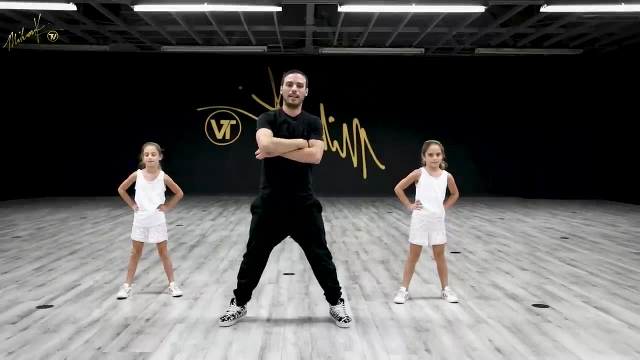 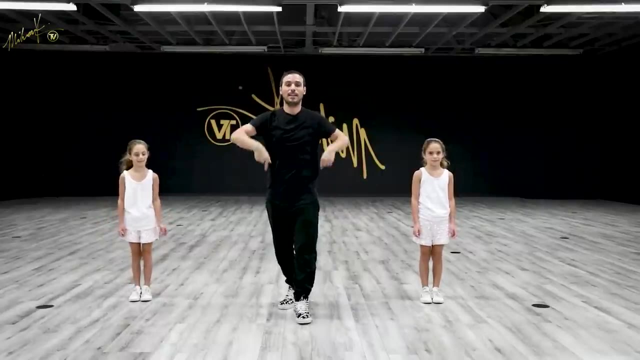 One, two, three and four and five, six, seven, eight, One. Nice, All right, Let's see if we can speed it up. How do you feel? A little faster. A little faster. Five, six, seven, eight, Down One. 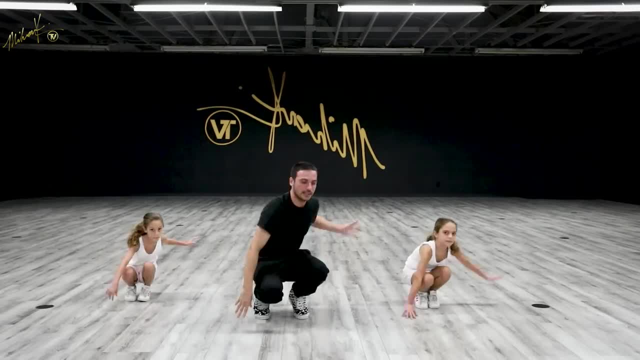 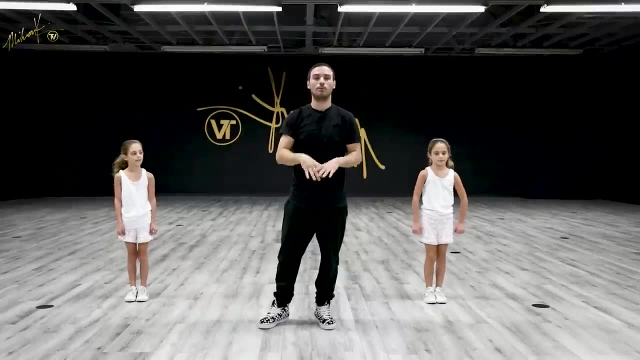 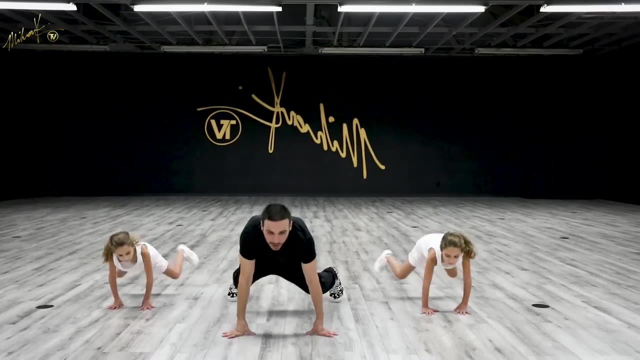 two, three and four and five, six, seven, eight, One. Let's do that one more time full speed, and then we'll try it with music. Only the second half. Okay, Just the floor. Here we go. Five, six, seven, eight Down. One, two, three and four and five, six, seven. 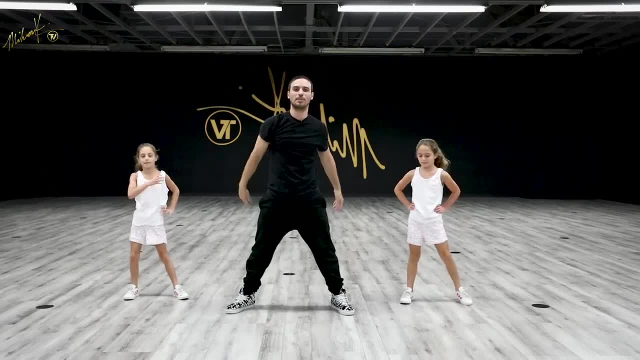 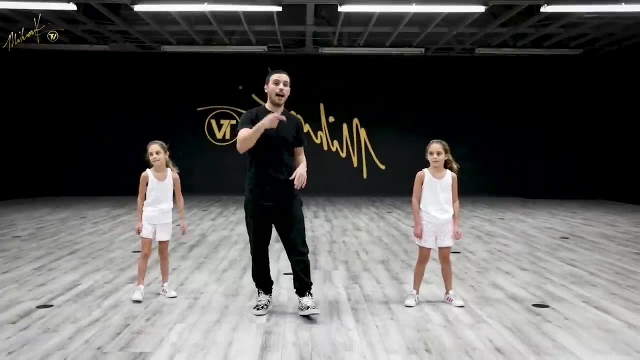 eight, eight, one, Awesome, Let's try it with music. Here we go. All right, here we go. Second half: only I'll count you guys in Girls ready: Ready, Five, six, five, six. 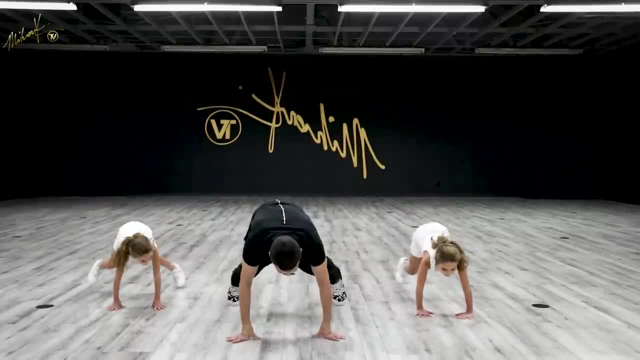 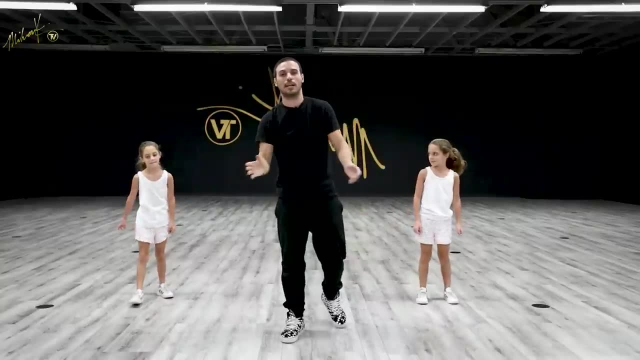 down to the floor. One, two, three and four and five, six, seven, eight, one. Good, Let's do it again. girls, Here we go. I'll count you in. This is five, six. 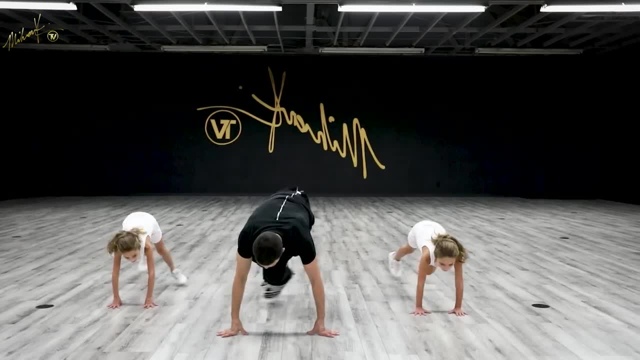 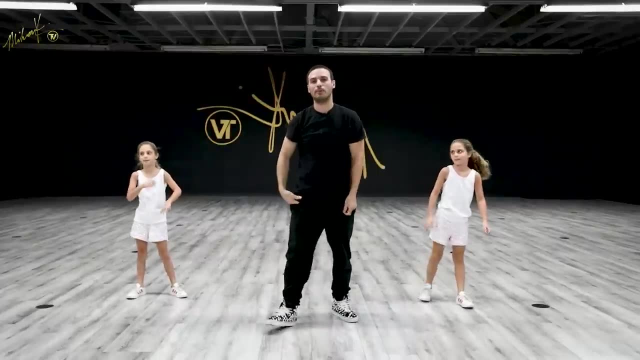 five, six down to the floor: One, two, three and four and five, six, seven, eight. Hold Good, Let's do it one last time. Here we go, And five, six, five, six. 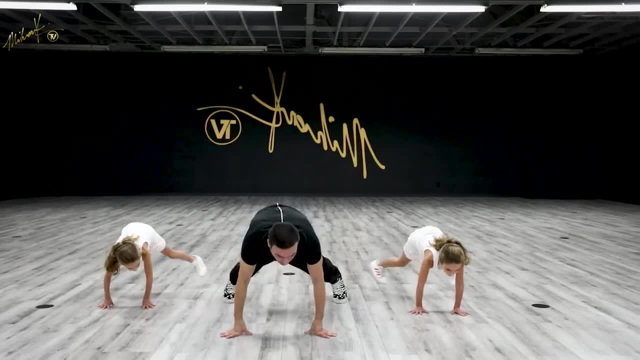 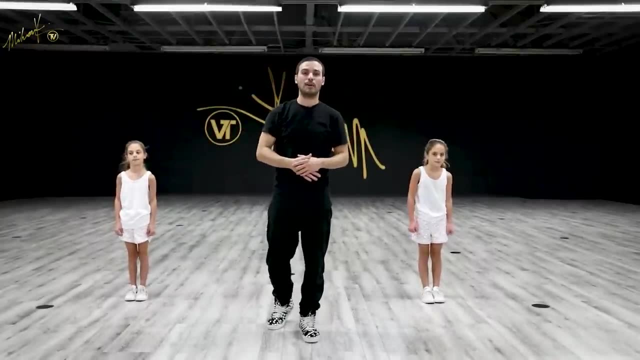 take it down. Go one, two, three and four and five, six, seven, eight, Hold. All right guys, that was awesome. Let's take it back to the very top. Walk it slow, Walk in medium tempo. 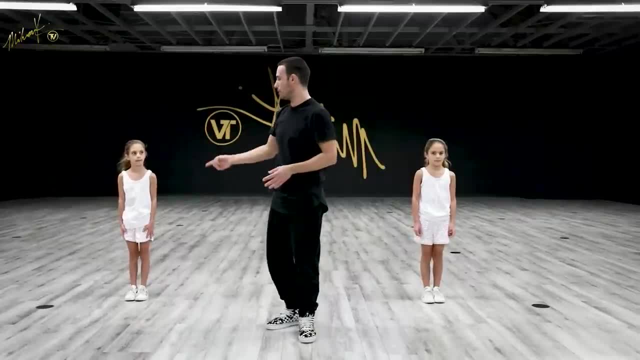 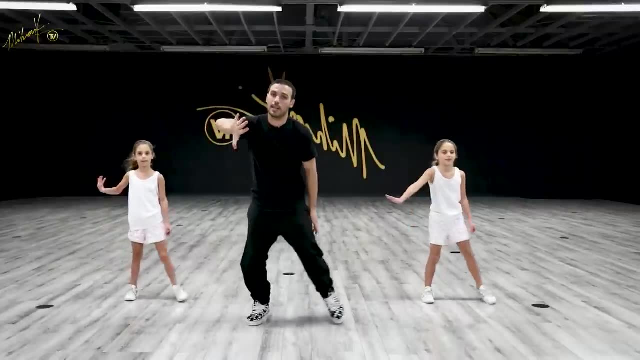 Walk in real tempo From the top and then we'll just dance it out with music. Girls. you ready, Ready? Here we go From the very top, slow, From the slide Six, seven, eight. slide One, two, three, four, five and six, seven, eight. 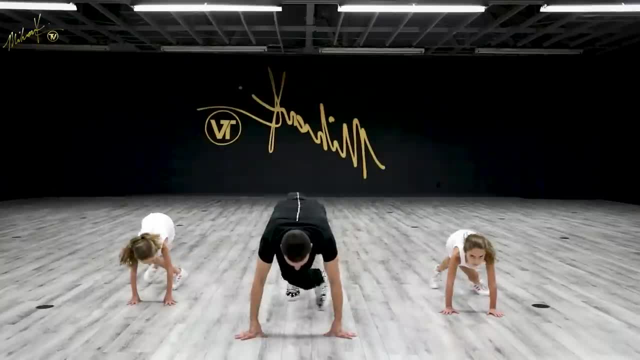 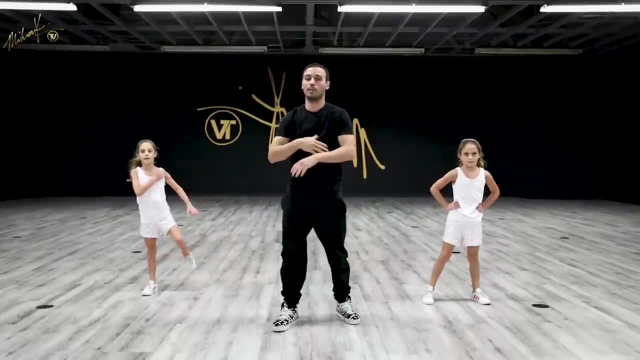 Down one kick, two, three and four and five, six, seven, eight, one. Good, That was pretty slow, So if you could do that, you're in a good place. So the next thing is just to review. 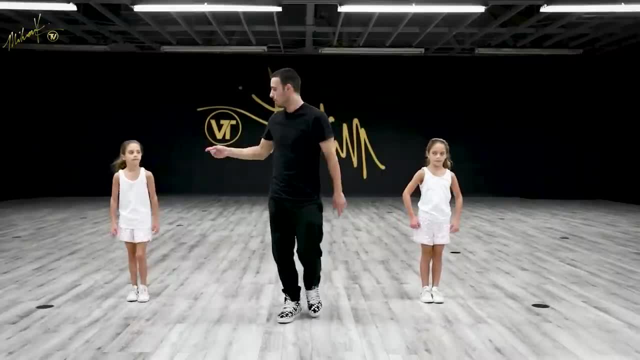 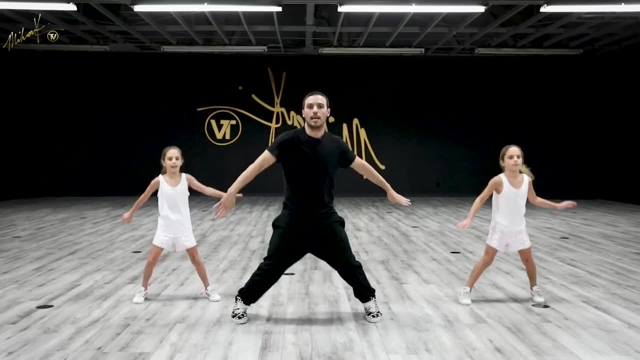 until you can catch up with tempo. okay, We're speeding it up just a little bit. Girls, here we go. Five, six, seven, eight, Slide one, two, three, four, cross and cross out hit. 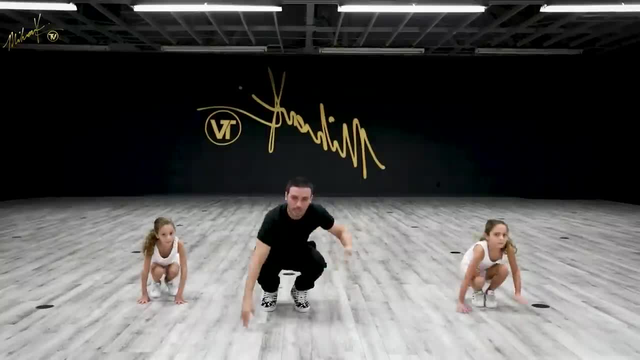 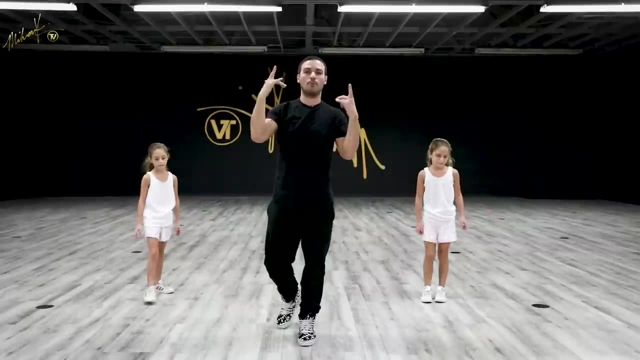 Down one, two, three and four and five, six, seven, eight, One. Good, We got one last time together. We're gonna do full tempo and we're dancing it with music Girls. here we go.